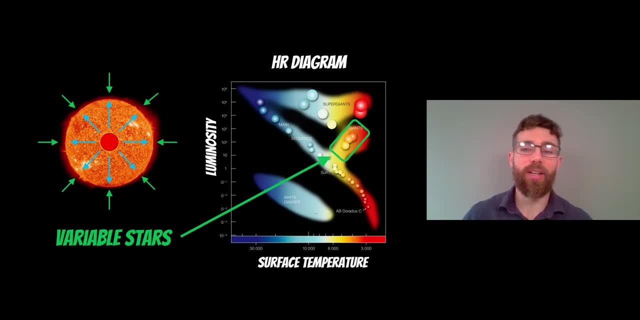 when they go to the upper right they become a giant star, so they actually kind of swell up a little bit. they swell up quite a lot and they actually begin to pull some of these stars. so Cepheid variables are the ones we're interested in for this and they may do something like this: 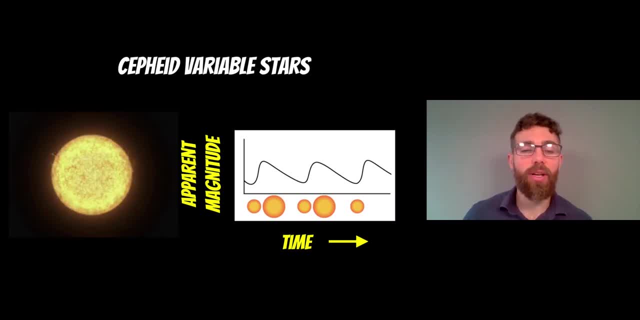 so they actually kind of pulsate or they change their brightness. so they get bigger, smaller. as a result of that, their surface temperature changes and their brightness will change. so their apparent magnitude as we observe them will fluctuate and it typically has a very regular pattern. so on the right you can see here, over time they're going to be a little bit bigger and 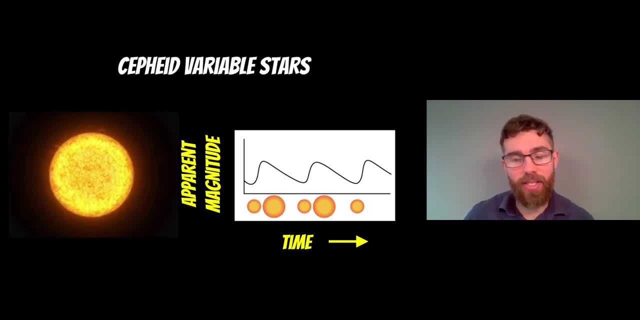 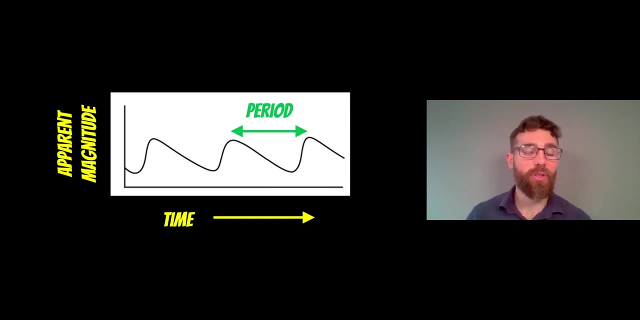 over time, as the star kind of pulsates or varies, we get this change in apparent magnitude, and it's quite a regular period for these particular stars. so it's a very useful thing. now we can get the period very easily. so if we just measure the apparent magnitude of that star, so the apparent 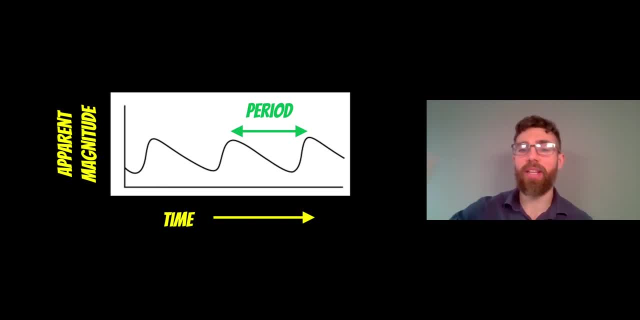 magnitude is how bright it appears to us from Earth and depending on its distance it will be brighter or dimmer. so if it's closer it'll be quite a lot brighter. if it's further away it will be dimmer. we can measure the apparent magnitude: how bright it appears to us and when we plot that against. 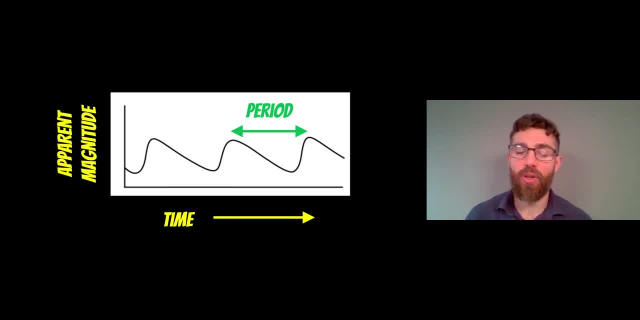 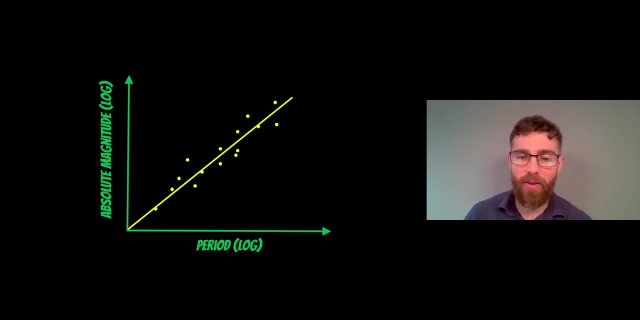 time. it's very easy then to get that period. so for example, here we're just going from peak to peak, we measure the time difference and we can then get the period of that variable star, and there's a particular relationship for these types of stars. so if you plotted the period against 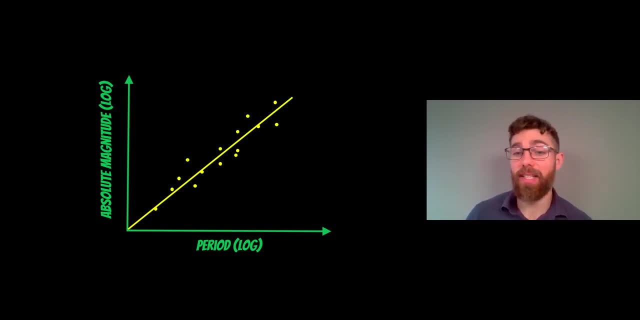 the absolute magnitude. so this is how bright the star would be from some set distance, so from the same distance all the time. that's their absolute magnitude. then they typically show this sort of relationship here, and this is a log, log plot, but we have this relationship. now we can measure the period. 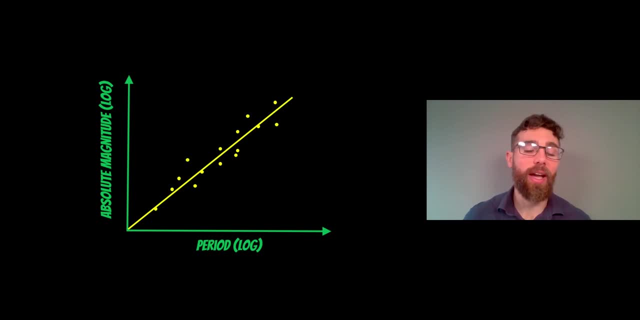 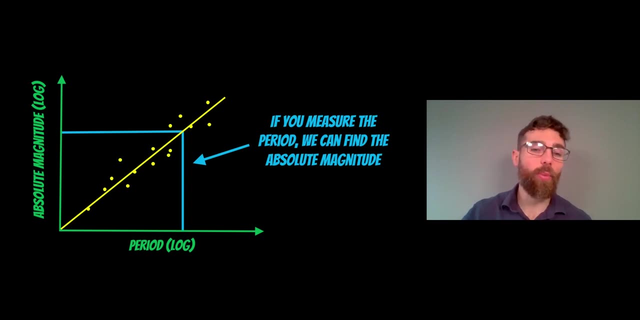 so before we saw the period of their apparent magnitude. so we can basically measure that. so let's say we have a period here. we then go up on the plot and go across. we can then get a value for its absolute magnitude. so we only need to measure the period. I know what top star is.